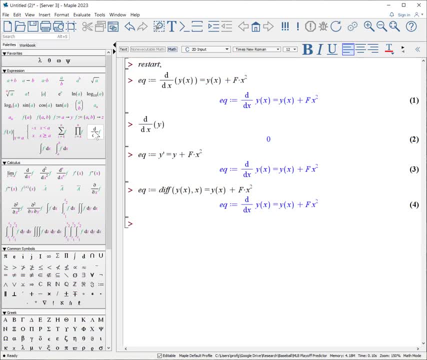 But I prefer the. either You can use the prime notation or using the palettes. The last way we can do something is to use the dot notation, For example. I'm going to make my equation Now. we're going to have X as a function of T. 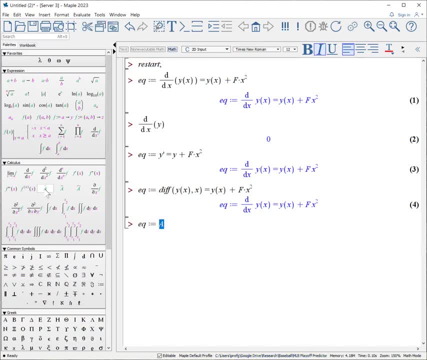 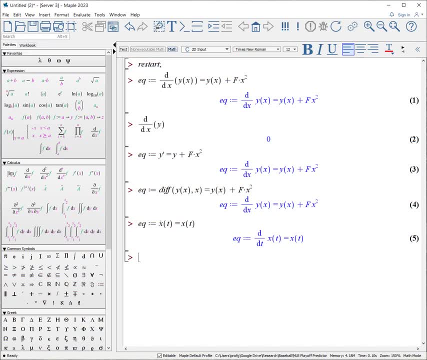 Equals X of T. Again, if you are using the dot notation, then it's going to assume that you're doing a derivative with respect to T. So if you say the same thing, EQ colon equals Select in the calculus palette the dot. 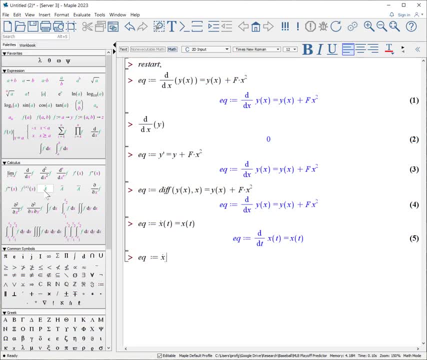 Put X. Right arrow. equals X equals X. It will substitute The function as a function of T. Anything that's beyond that requires just choosing one of the other palette characters. here, For example, what if we have a second order differential equation? 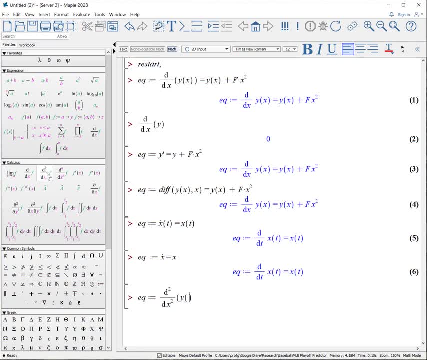 So I'll select the second order with respect to X of Y of X Plus the first order with respect to X. Tab: Y of X Plus Y of X equals zero, And that's how you enter your equations. And that's how you enter your equations. 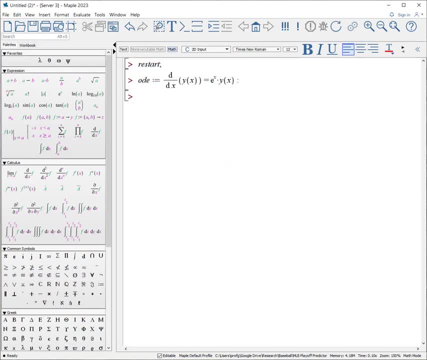 Now that we know how to enter our ODEs, now it's time to solve the ODEs, And the function or procedure that we need to use is DESOLVE. So here's our ODE that I've created, And now I'm going to apply it to DESOLVE to get a solution. 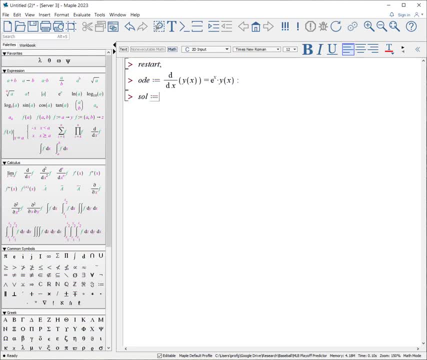 Again, good practice is to assign the result to a variable, So solution is DESOLVE. And then we put in our ODE, Since there's really only one variable, that is the derivative, For which is the only function. that is our equation. 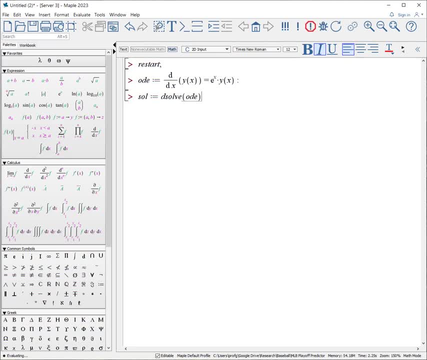 It will immediately sort of get. look for the solution to Y of X. It returns the answer And in fact it returns the answer with a constant. Notice the constant is C1.. This shows that it is a family of solutions, Because we have not given it any initial conditions. 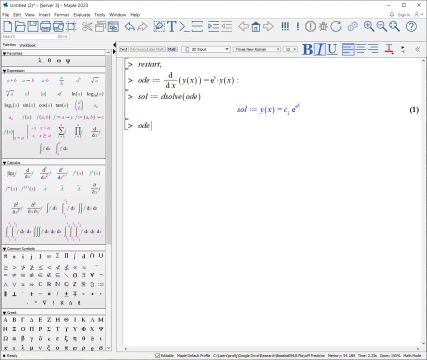 No conditions whatsoever. Let's try another one. ODE colon equals- I'll use the prime notation- X times Y. I prime minus 2 times Y equals X squared. Put a semicolon. Show that. this is what the equation looks like. 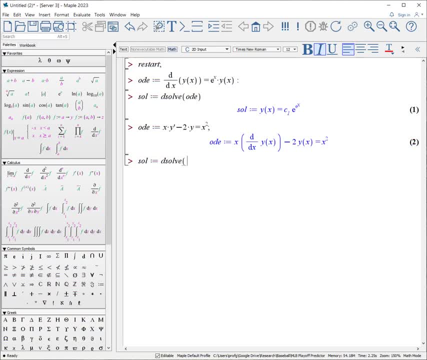 And again solution: DESOLVE ODE And it returns a solution. Again, it will include a constant, Because this is a first order ODE And we have not included our condition. We can create a second order ODE as well. 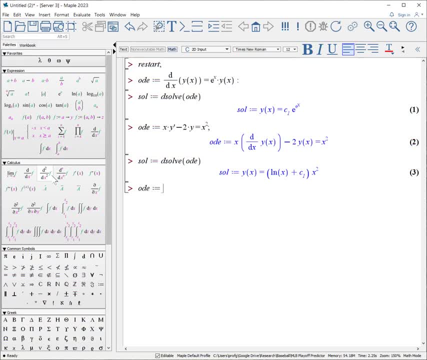 ODE colon equals- I'll use the derivatives here: With respect to R of Z of R, Minus 6 times the derivative. First derivative: With respect to R of Z of R. Some people have asked me: do I really need the parentheses? 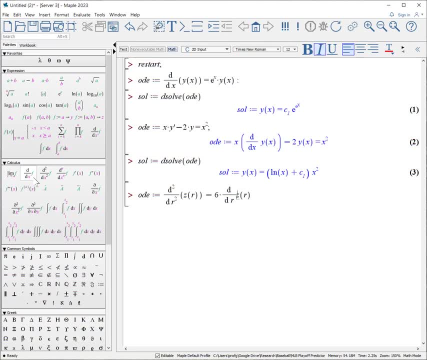 And the answer is no. You can remove those parentheses And it will recognize it correctly. Plus 5 times Z of R equals 0.. What does the equation look like? Again, there's the derivative. we expect Solution: DESOLVE ODE. 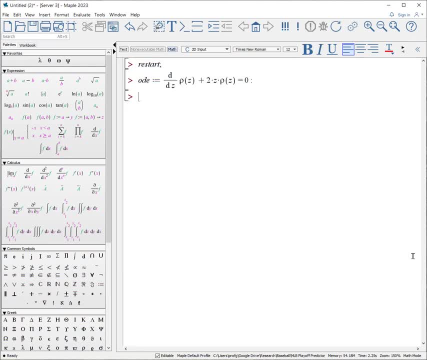 And again, it will know to solve for Z of R. What happens if your ODE does have a condition, Or maybe a bunch of conditions? How do you include that into your DESOLVE? Well, DESOLVE expects either a list or a set of solutions. 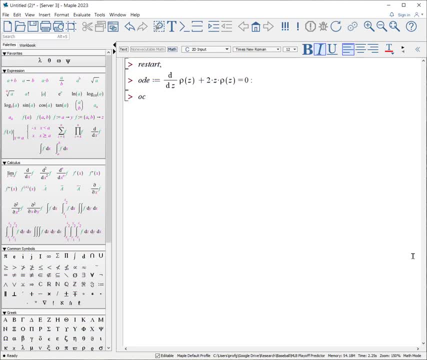 So here's our ODE, And what we're going to do is we need to create an initial condition equation, And I'll say row of 2 is equal to minus 1.. Okay, So we are ready to create our solution: DESOLVE, DESOLVE, curly brackets to save a set ODEs and ICEs. 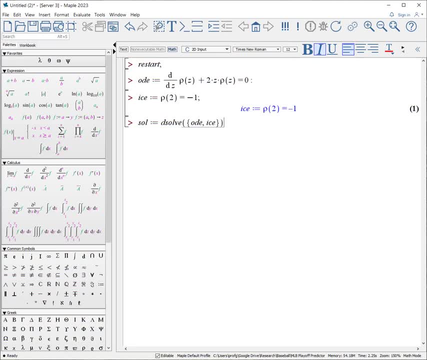 And when you do, it knows that the only variable it has to solve for is row of Z, And what it does, it produces the correct results. But you've got to be careful, because if your math doesn't make sense, Maple cannot solve it. 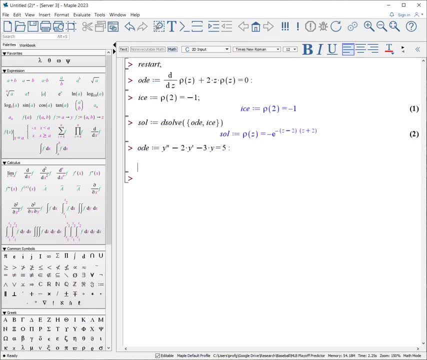 Okay, Let's do another example, And in this example we have a second order ODE. Therefore, if we're doing an initial condition equation, we need two initial conditions. So I will use the two initial conditions ICEs, two initial condition equations: colon equals. 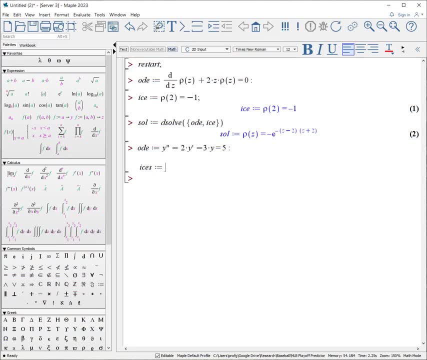 And then I need to just list- actually in a sequence but not put them in a list- the two equations, For example, Y of zero is equal to zero And Y prime of zero is equal to one. Okay, Again, Maple will recognize. and let me show you what Maple thinks about this. 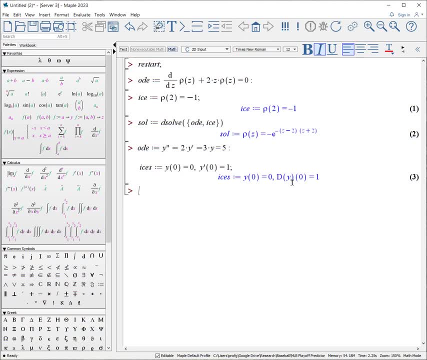 It says, okay, it recognizes that Y of zero is equal to one. And then it says I'm going to need to do a derivative of Y and evaluate at zero and assign that equal to one. So that's what the big D stands for. 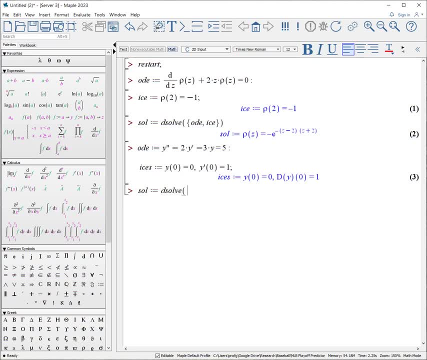 All right, We're ready to solve. DESOLVE curly bracket. Our ODE is one, One of the equations, And then the ICEs are two additional equations. Close And it returns a result. Okay, You've been able to write your ODEs and your conditions. 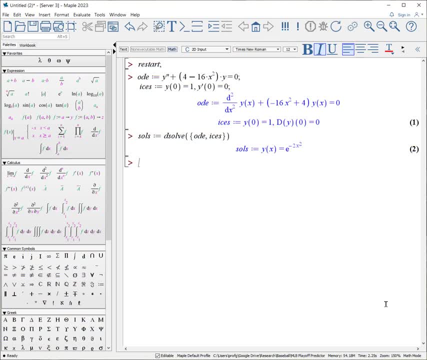 You've been able to solve your problem. How do you extract the solution? My recommendation is to use EVAL the procedure. In addition, I also recommend not assigning the solution to the variable itself, So I will create Y underscore. underscore: SOL- right arrow colon equals. 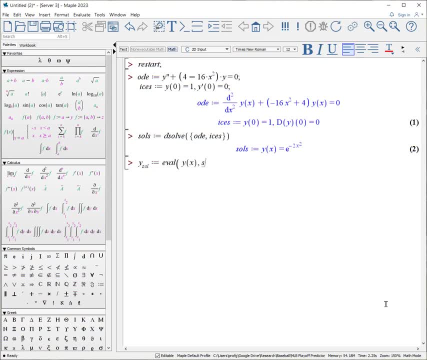 I'm going to evaluate for Y of X. given my solutions, It will extract it out. Now I have the expression called YSAL. If I want to make a function out of it, I can do Y underscore, underscore, SOL, right arrow, colon equals and make function. 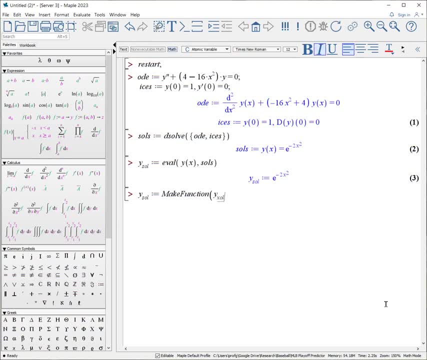 If I want to make a function out of YSAL comma X and now it is a function of X At this point, now we can actually start plotting it. For example, I want to plot YSAL of X from X equals minus 10 to 10..